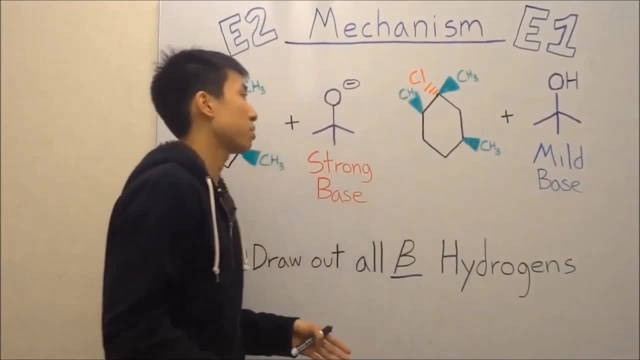 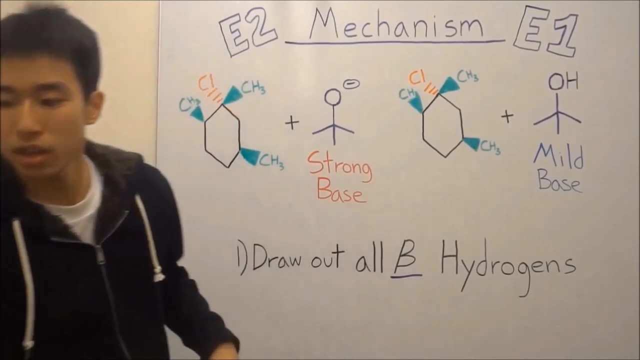 these methyl groups over here that are slowing it down and preventing it from getting through to your carbon. So we're not going to be doing a substitution reaction. Another way you could think about it is: imagine if I was the nucleophile and I had three of these backpacks on right. 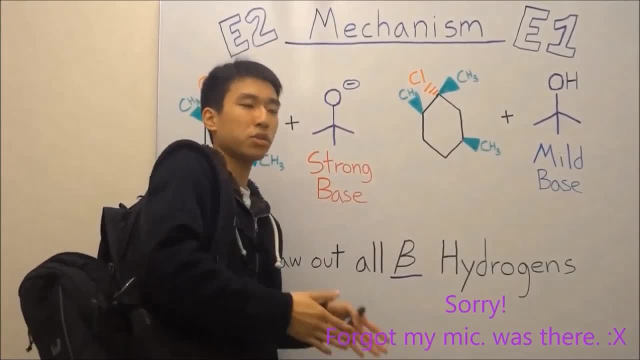 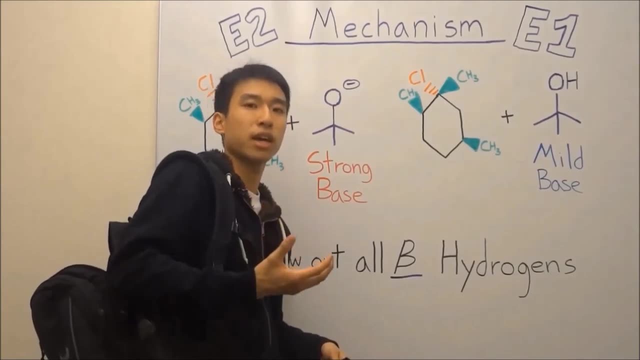 I had one over here, one behind me and one to my left. If I was trying to go through a narrow doorway right, I can't get through it because these backpacks will be blocking. I guess you could think of it as the backpacks will be slowing me down. one. 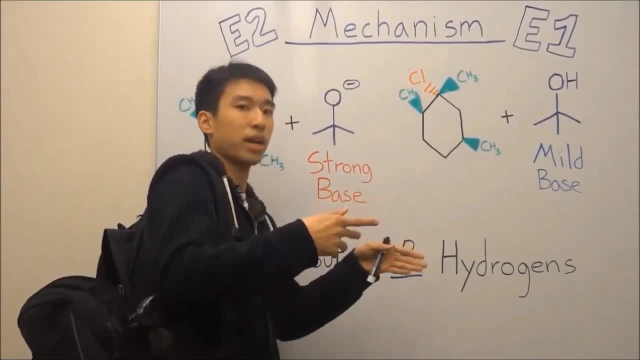 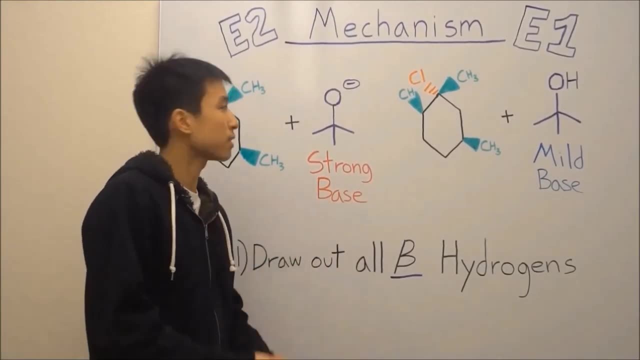 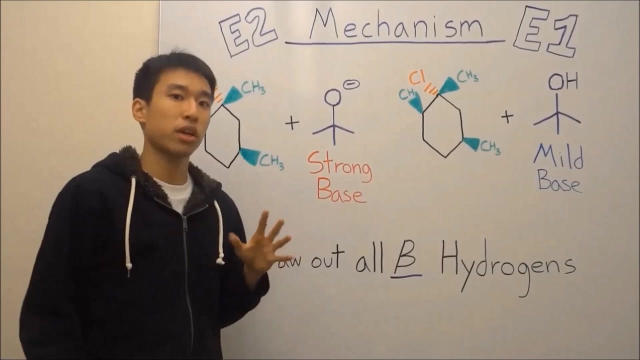 And two, they're going to make me too wide to go through the doorway, And that's exactly why These nucleophiles here don't act as nucleophiles and they actually act as a base. Okay, So yeah, for E2 you want a strong base, since E2 means that two molecules are going. 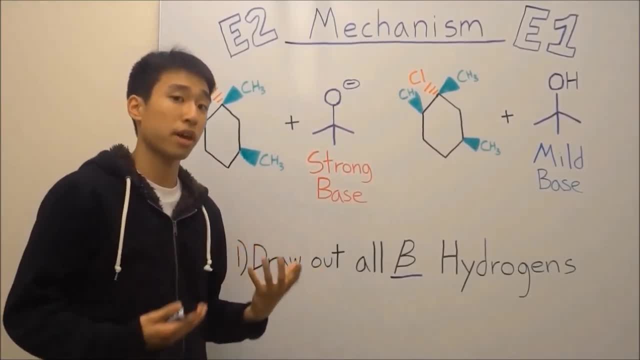 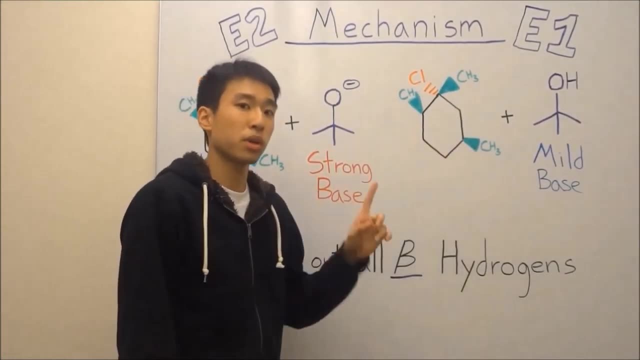 to have an effect in how fast the reaction occurs. So both molecules need to be reactive. but E1, all you need is a mild base, because only one molecule is going to have an effect on how fast the reaction occurs And that's not going to be your base. It's not going. 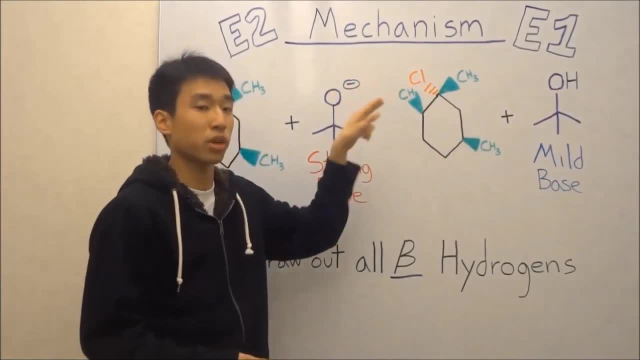 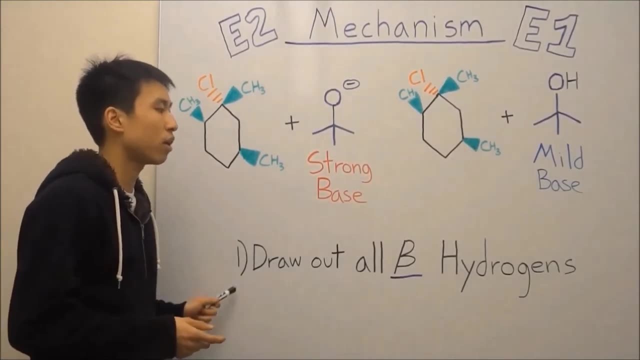 to start the reaction. It's going to be your substrate here, with your leaving group chlorine. All right, so let's get started then. The first thing you want to do for elimination reactions is draw out all your beta hydrogens. In case you guys don't know what a beta hydrogen? 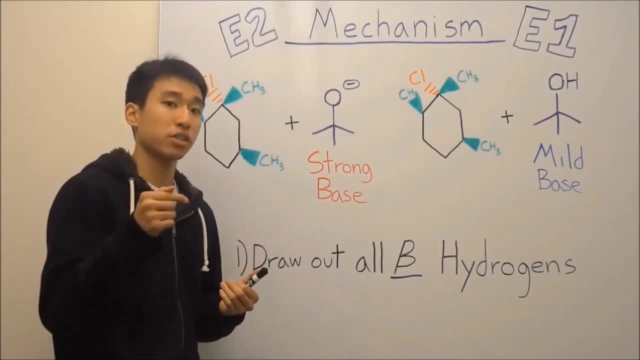 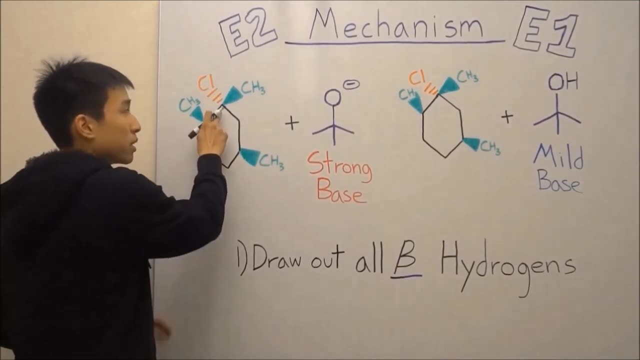 is. it's basically the hydrogens that are attached to your beta carbons. So let's find our beta carbons in our substrate first. So if you look over here, right, this carbon here, this one- it's not going to be a beta carbon because it's the first carbon that's. 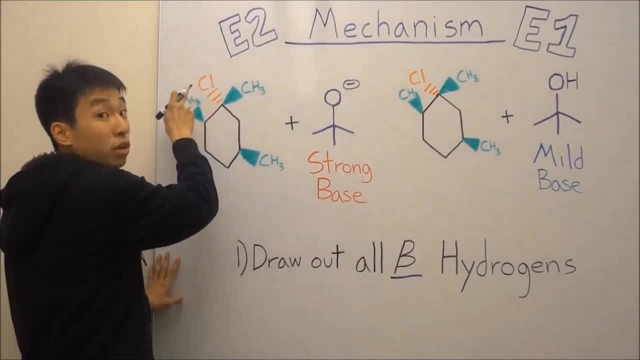 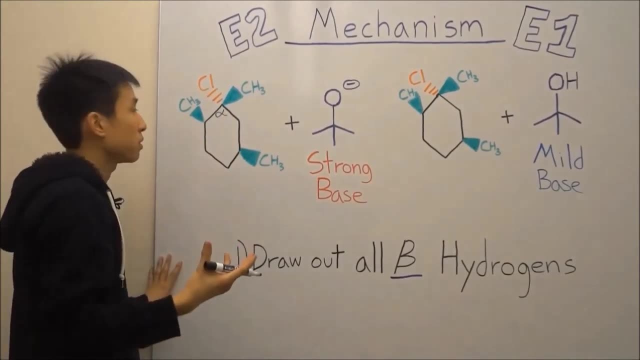 attached to your functional group or your leaving group, the halide chlorine. So this is what we're going to be calling an alpha carbon. Okay, So your beta carbon is going to be the next carbon, That's one carbon away from your alpha carbon. So you have one beta. 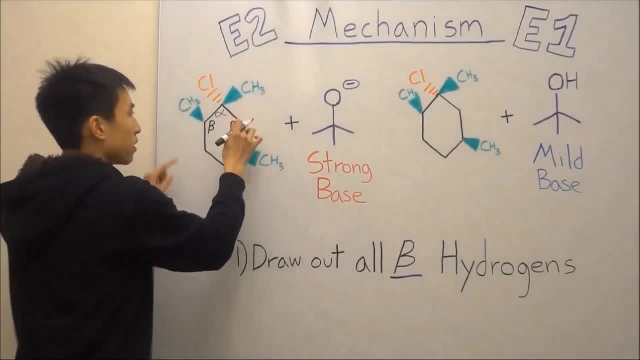 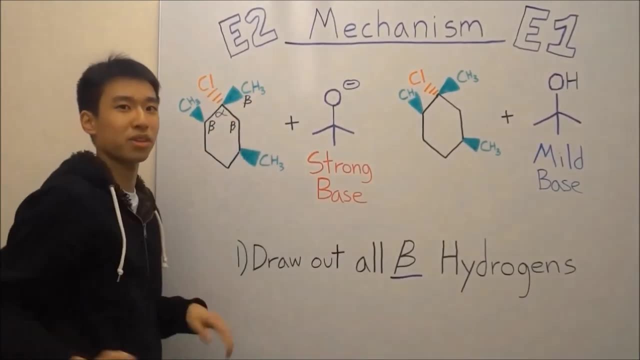 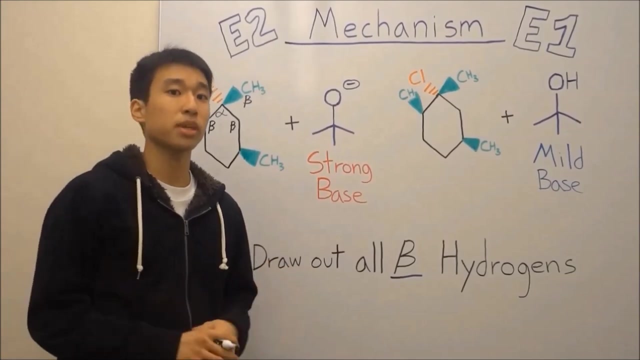 carbon over here, one beta carbon over here- Right, These two guys- and one more beta carbon up here, because they're all one bond away from your alpha carbon, All right. So the same is true for this molecule over here. So I want you guys to take a second and just draw out all your beta hydrogens first, because 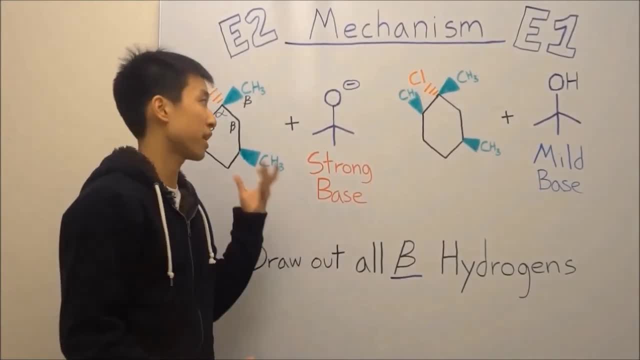 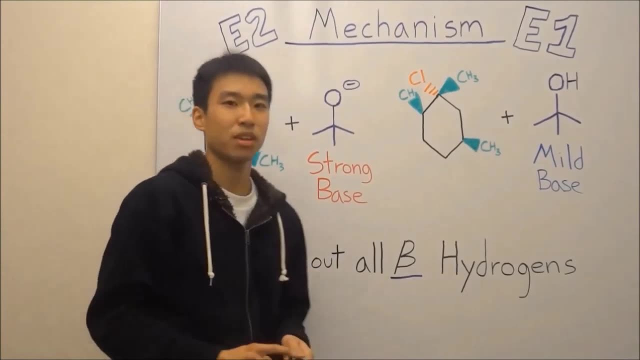 that's what your strong base or your mild base are going to be reacting with in your reaction here. Because if you think back to gen chem, right, what do bases? do Bases grab protons or hydrogens? Okay, Take a second. okay, And pause the video. Okay, All right. 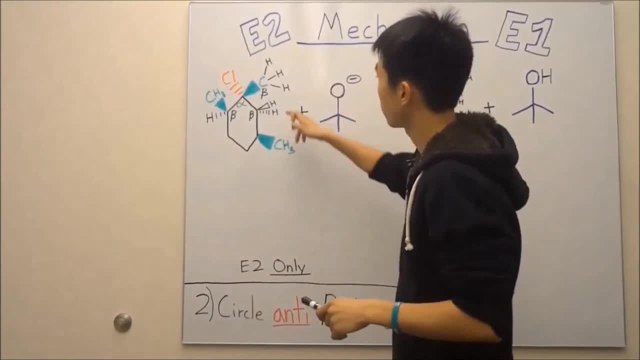 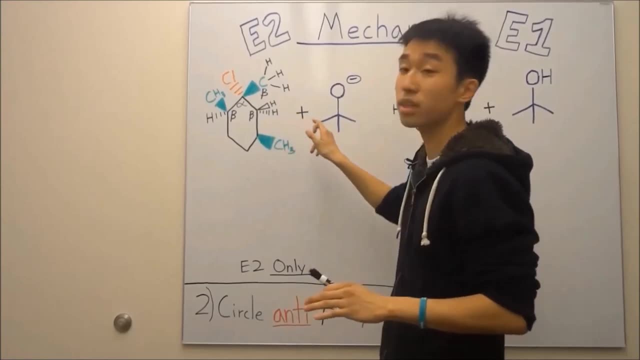 Okay, So this is what you guys should have gotten. okay, Your beta hydrogens should have been here, here, here, here, here and here, So you should have a total of six beta hydrogens on both substrate that you draw. now. The most common mistake that people tend to make is: 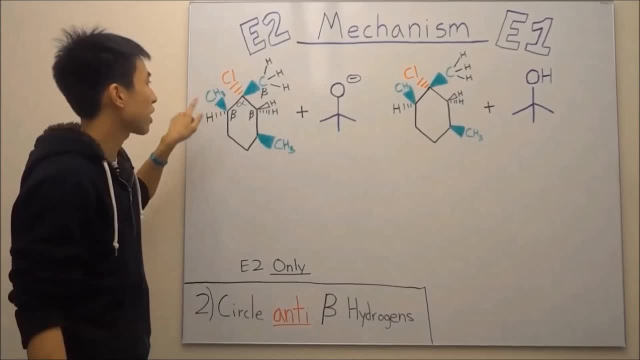 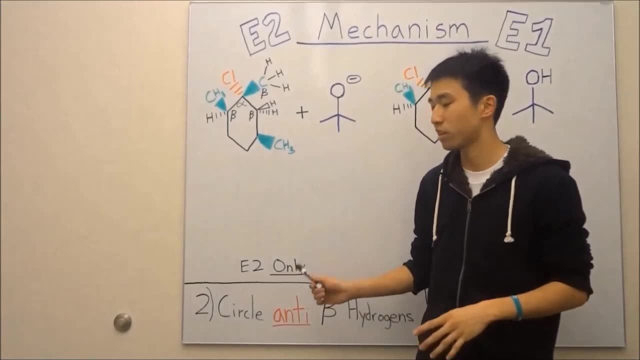 they draw out the hydrogens on this carbon over here, because it kind of looks like this carbon is beta, but it's actually not, So don't worry about it. So the next step that you have to do is to draw out- oh sorry, not draw out circle. 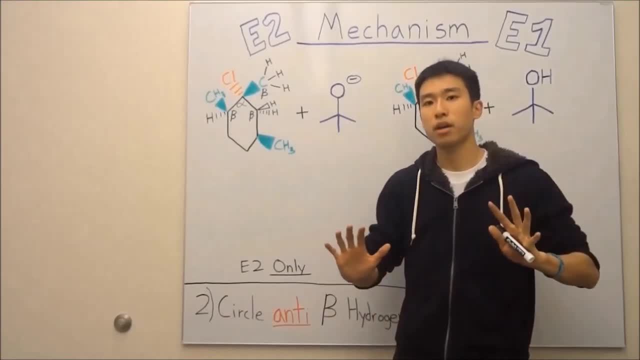 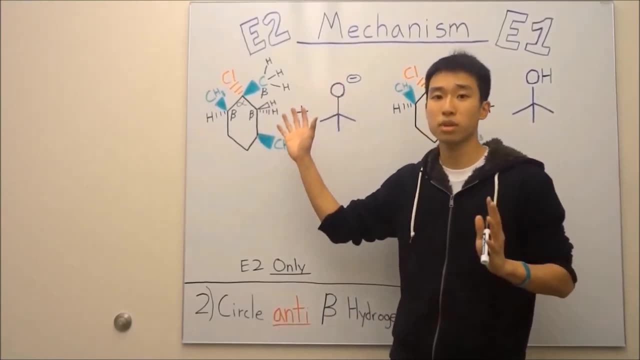 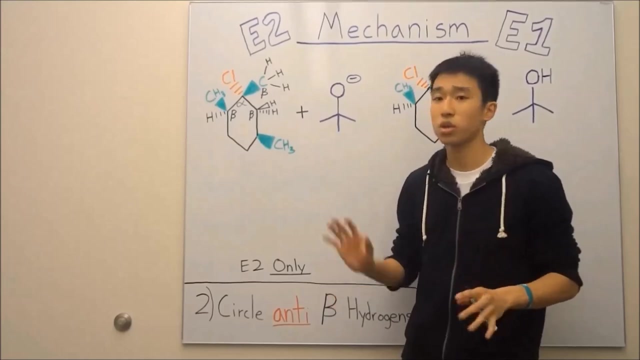 here, And the reason for that is because, well, first of all, different professors teach E2 elimination differently. A lot of professors- and my professors. they taught me that E2 elimination can only occur at the anti-beta hydrogens. The reasoning behind that I'll show you guys. 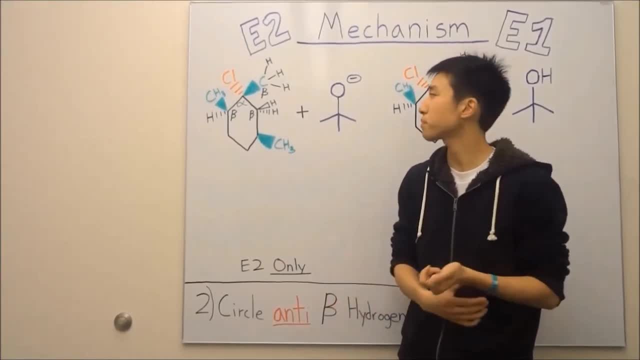 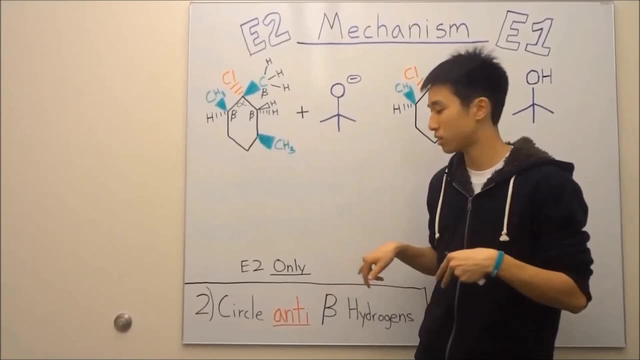 later, but it's just more stable and faster. But I read online recently that some people say that syn elimination can occur, So elimination with the syn beta hydrogens. But that all depends on your professor and how he teaches it. So make sure you guys double. 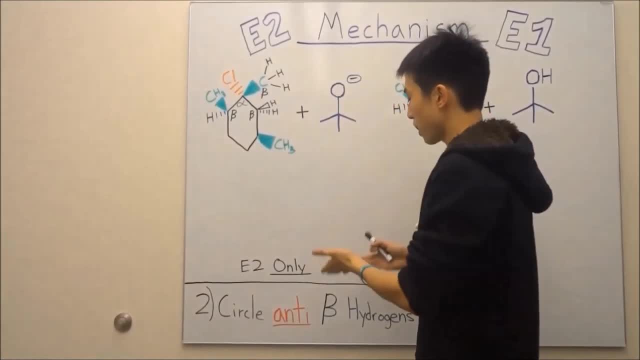 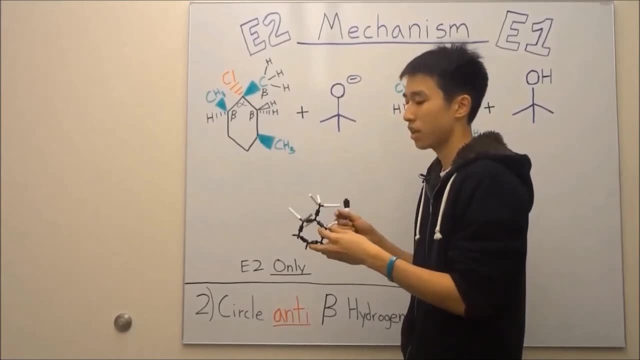 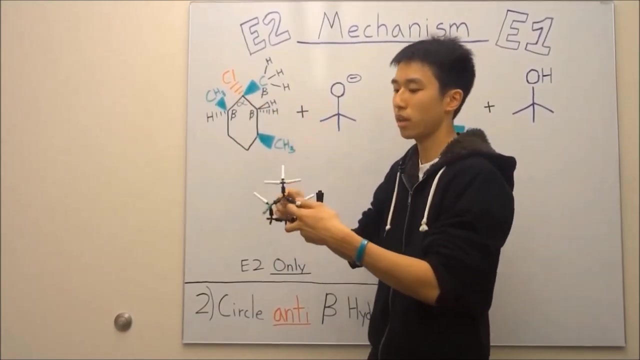 check your notes, okay. So, anyway, what I mean by anti-beta hydrogens is hydrogens that are on the beta carbon and that are opposite of your leaving group, chlorine. So chlorine is dashed over here, right? So that means that it's going into the board like the model. 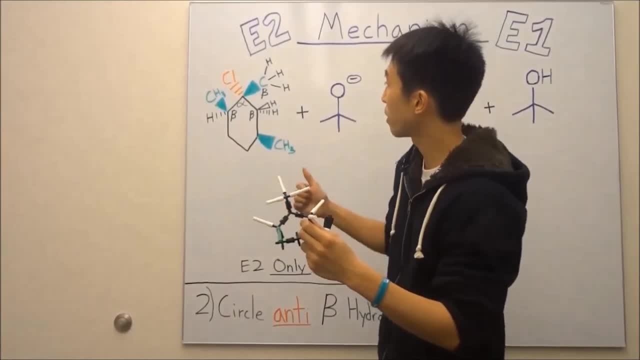 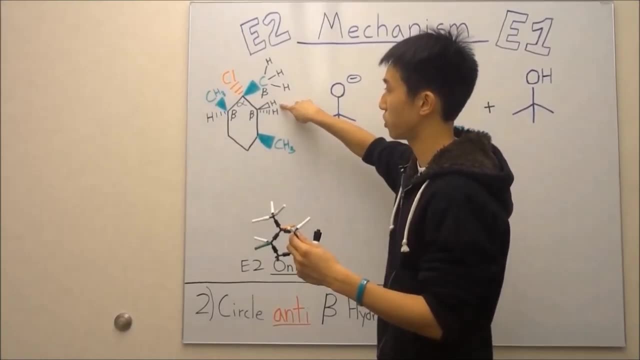 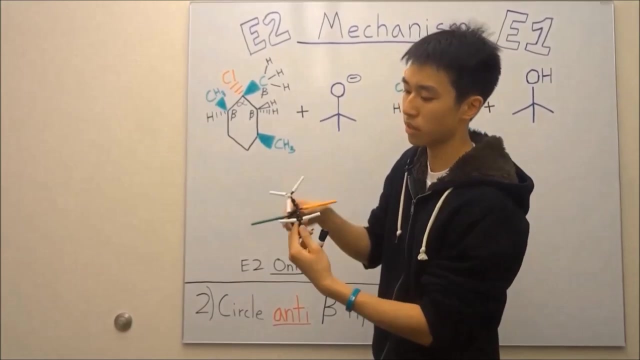 right here. See how chlorine's going away from you And then so anti would be a hydrogen, so an anti-beta hydrogen would be like this hydrogen over here. It's wedge, so that means it's coming out at your face. So that's this hydrogen over here, okay, So these guys are 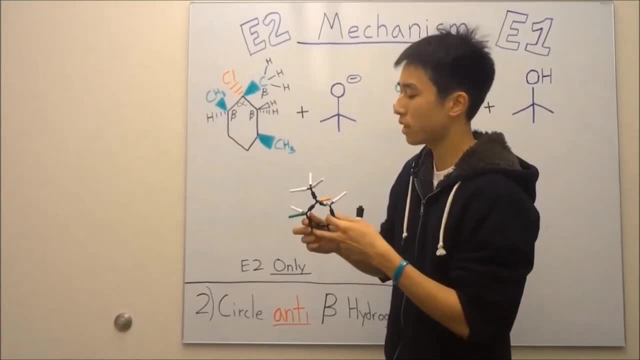 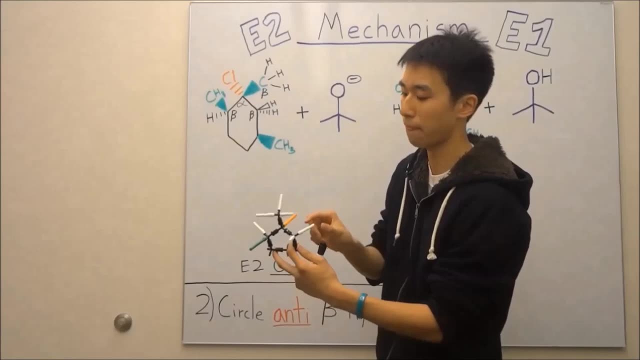 anti. See how they're facing opposite ways. But a syn hydrogen would be this hydrogen over here, the one that's dashed, Same thing as your chlorine, because it's facing the same side. all right, And can you find the other syn hydrogen? It's right over here.